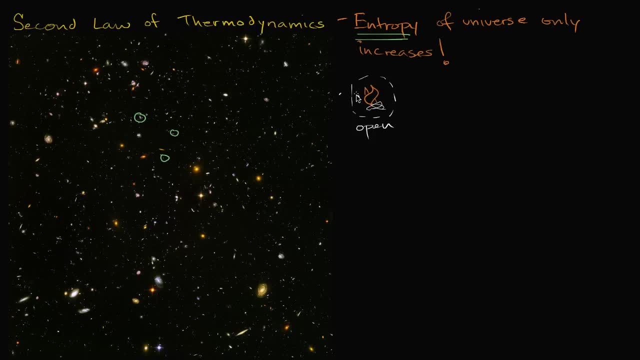 It's releasing heat. it's warming up the air molecules around it. it's releasing light out into the universe. There could be interactions from the rest of the universe into the system. so it isn't isolated from the rest of everything else, But a closed system. it is isolated. 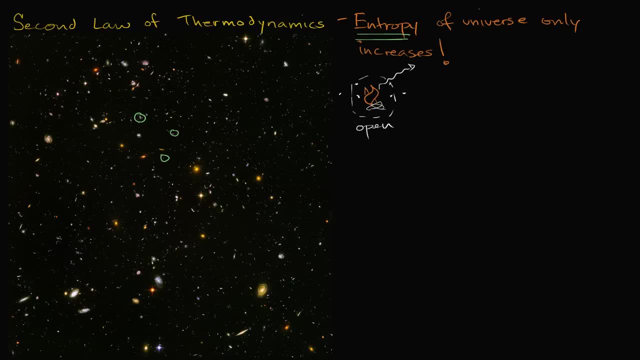 And it's very hard to create a true closed system in our everyday life, but we can approximate it, And the one that you've probably experienced in the not too distant past is an ice cooler In an ice cooler. we're at least attempting. 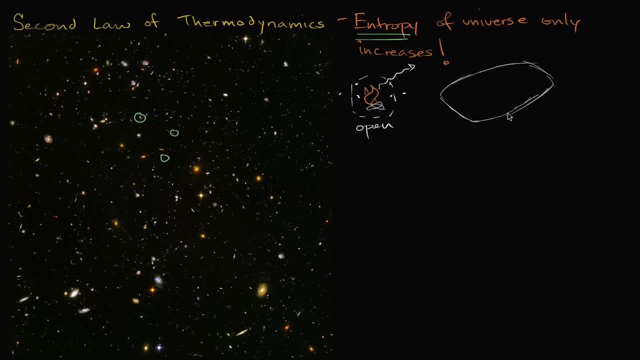 to thermodynamically isolate the inside of the cooler from the outside, from the rest of the universe. So this is, and the way we do it is: we have some type of an insulating material, maybe some styrofoam, and we could put and we'd use it to maybe store ice. 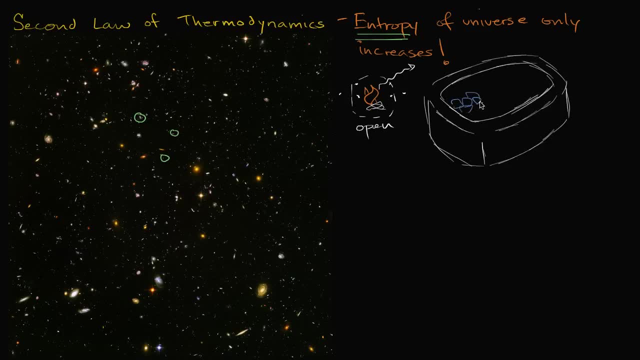 But it's not a perfect closed system because eventually the heat from the rest of the universe will warm up the walls of the cooler and eventually that heat will warm up, will be transferred to the ice and it will warm it up and it will and it will melt it. 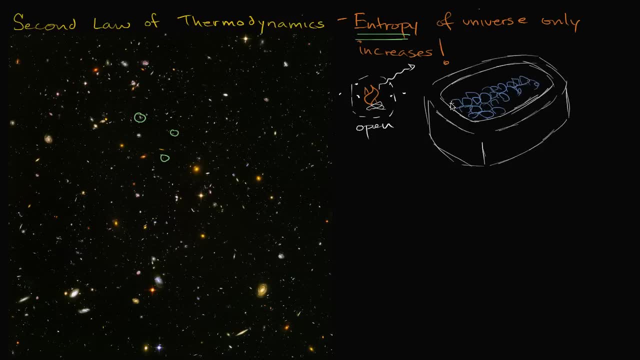 So it's not a perfect closed system, but it's a good approximation because we're at least attempting to isolate it thermodynamically from the rest of the universe, And I can even make a little cover of this, just so that we really wanted to isolate it. 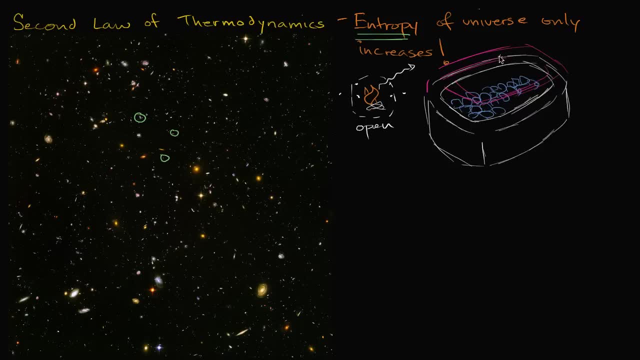 And in research labs you'll see things that are much better approximations of closed systems. but even those, at some level they're going to interact with the rest of the universe, The ultimate closed system. so this is a closed system. 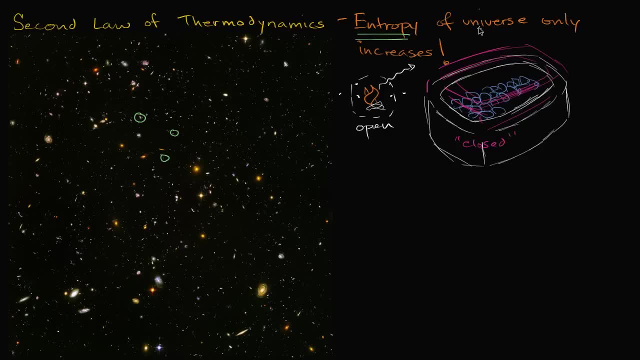 is really? is really the universe, Nothing to interact with outside of it, thermodynamically or thermodynamically. So let's think a little bit about this definition. The entropy of the universe only increases. Why does this make intuitive sense? Well, the best example I can think of: 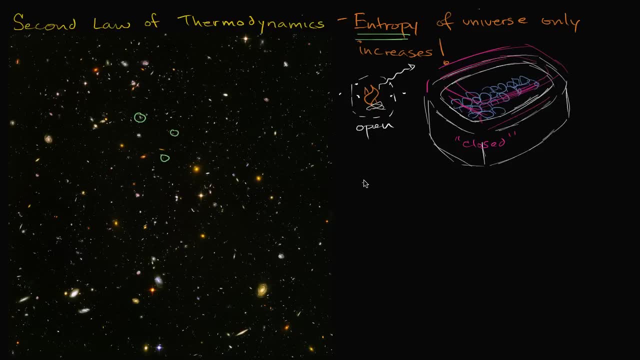 is just straight up diffusion. So if I were to have, let's say, I have a container, so I have a container and I'll make it a, I'll make it a closed container, I'll we'll say this is some type of theoretical. 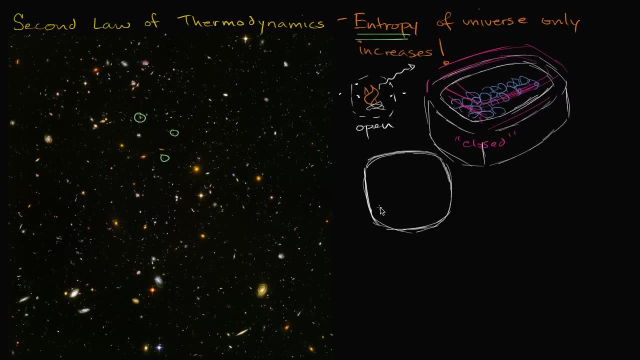 ideal closed system here. And let's say I had some ideal gas, Some ideal gas molecules right over here. They have some average temperature, but that means they all each have their own individual, their own individual kinetic energy. They're all bouncing around in different ways. 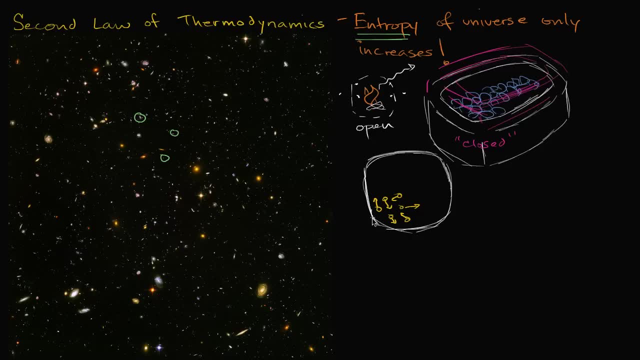 What's going to happen over time? Well, over time- the ones on the left here- they're going to bounce off this wall and then they're eventually going to go in this direction, And so, over time, you're going to have a situation. 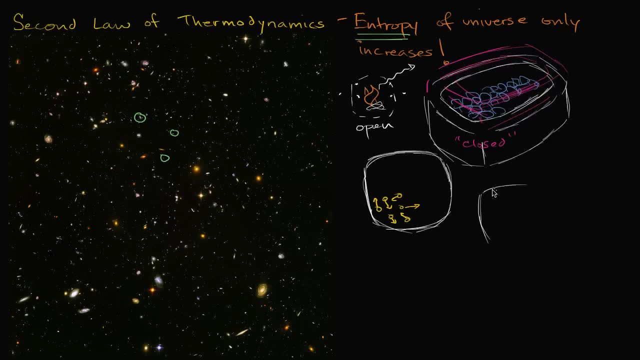 where the system is going to look something more like this. So the system is going to look more like this. Let's see, this is six particles. These six particles are going to diffuse throughout the container. So they're going to diffuse throughout the container. 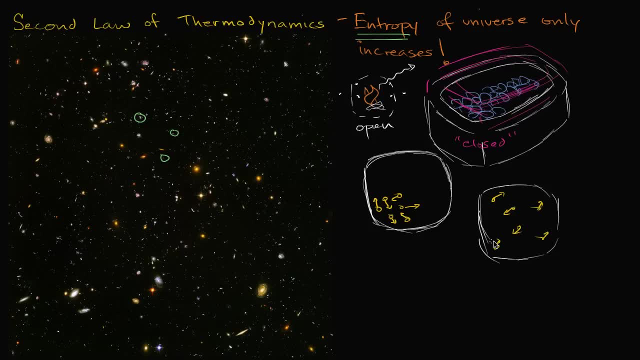 They're going to take up. they're going to take up more of the space of the container. Now, what just happened in that process? Well, when you knew that the particles were confined to this little section of the container, there were fewer possible states. 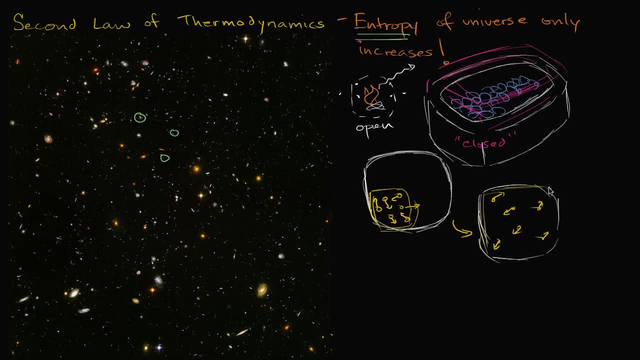 You had lower entropy than when you are here, When you know that it's filled up the container, there's more possible locations, more possible orientations for it, And so you're going to have more states. You have higher entropy, Higher, higher, higher entropy. 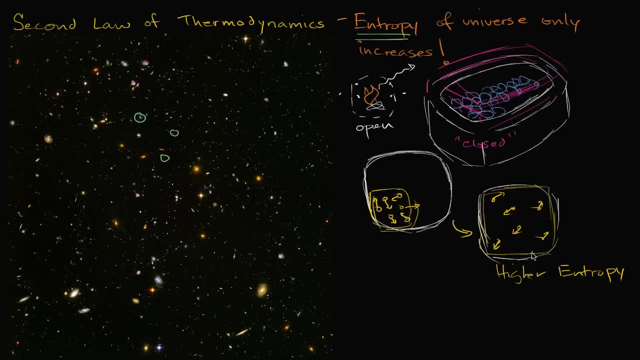 And, in general, these processes where you have the entropy increasing. we call these irreversible processes, Irreversible, irreversible processes. And why is it irreversible? Well, there's some probability that these molecules might just gather back into this corner of it, but it's very, very low probability. 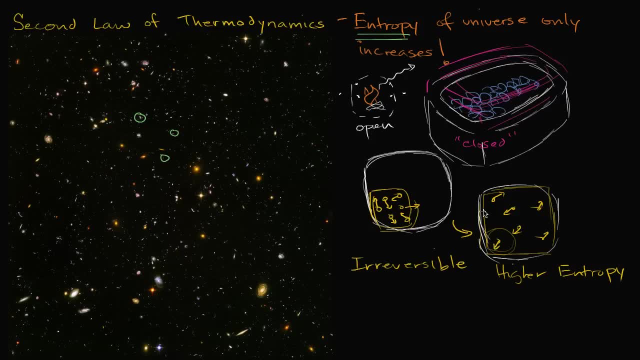 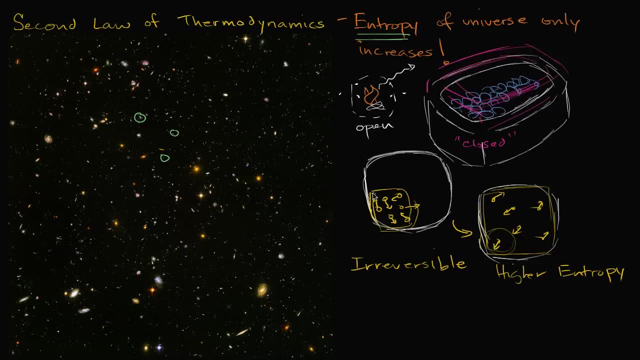 And there it's very unlikely that they just all bump together in the right way to start taking a smaller volume when they could actually fill the container, And so that's why you don't see. you know, smoke just naturally turn into some type of shaped particle or take up less space. 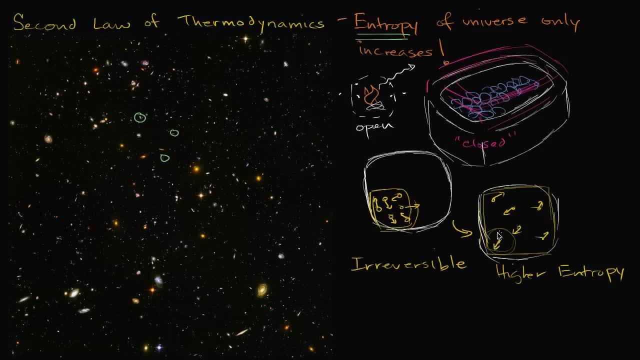 as opposed to filling its container. So this is irreversible, because you went from fewer number of potential states in the smaller volume to a higher number of potential states, And the universe is constantly doing this. That's why the entropy of the universe is only increasing. 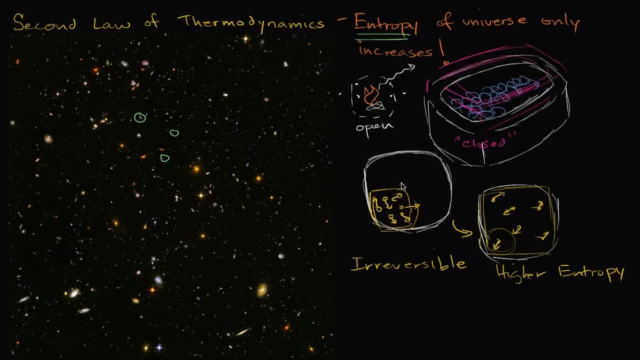 Now there's some processes that it feels like the entropy isn't increasing that much. So if you were to take one billiard ball right over here and you were to roll it into another billiard ball right over here and transfer the momentum to that one, 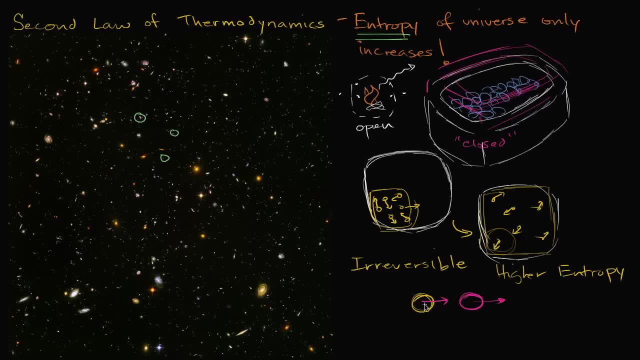 it feels like that could go the other way around, Like that other billiard ball could hit this one and go backwards. And at a macro level, it feels like this is a reversible process And people will tend to call this reversible, But if you really were to go on a microscopic level, 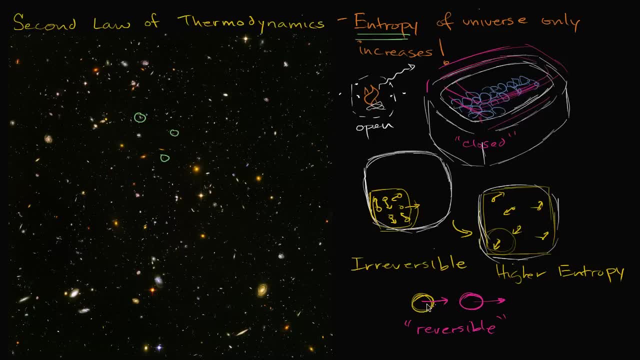 and it looks like the entropy isn't increasing that much. but if you were to look at it on a microscopic level and just to be clear, the entropy when this ball is moving and this is stationary, going to a state where this is moving, 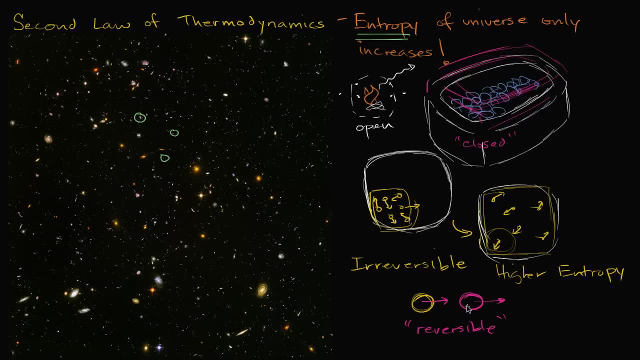 and this is stationary. it doesn't look like the entropy is increasing that much, And so that's why they tend to call this reversible, because you tend to observe things where maybe this one, it could go backwards, This could hit this one, and then this one could go. 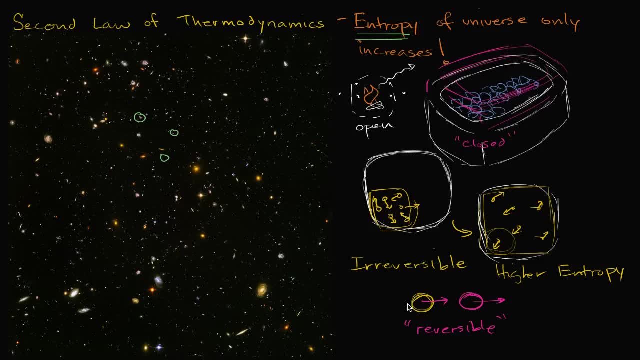 you can kind of run the film and rewind. But even there, if you were to look at a microscopic level, you would see that some heat is being generated and then some molecules in the ball are getting excited as they collide and as they have friction with the air. 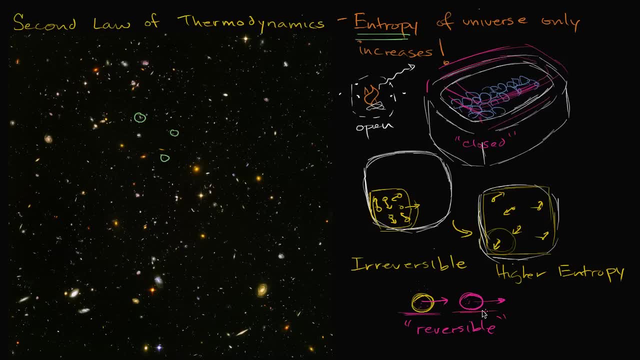 and as they roll on the ground over here, And you're never going to get those molecules to go back into the state that they were before that, you actually do have the entropy increasing in the system. So even when in our everyday lives, in thermodynamics, people talk about reversible processes, 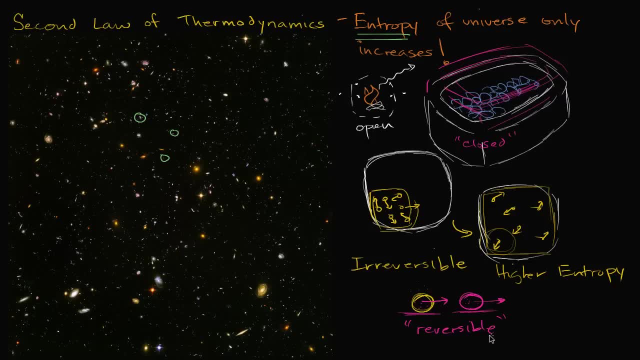 they're only approximately reversible, in that the entropy is only increasing a little bit. It's not like there's zero increase in entropy. Irreversible reactions: these are the ones- diffusion is a very obvious one- where it's very clear that you have an increase in entropy. 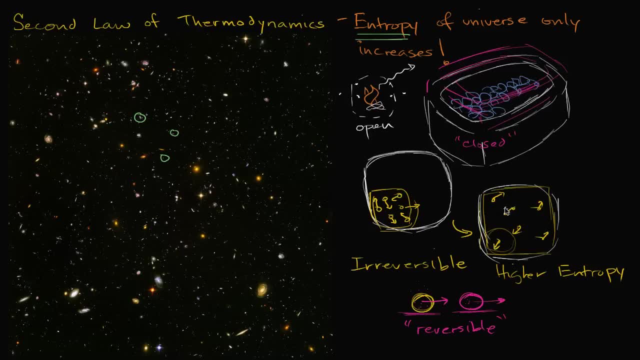 and it feels like it's a very, very low probability, or almost zero probability, of this thing ever going back to where it was. And you won't observe it, because when you're talking about that many molecules- something with 20 or 30 zeros of molecules- 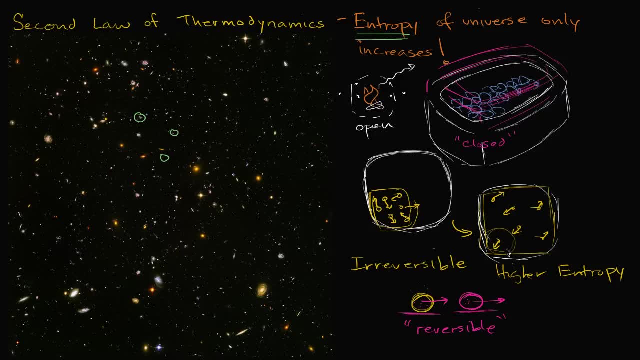 the odds of all of them just doing the right thing. you could wait around a very long time and never actually observe that happening, And so hopefully this makes sense that the disorder, in this way the number of states, only increases as you have more and more interactions.